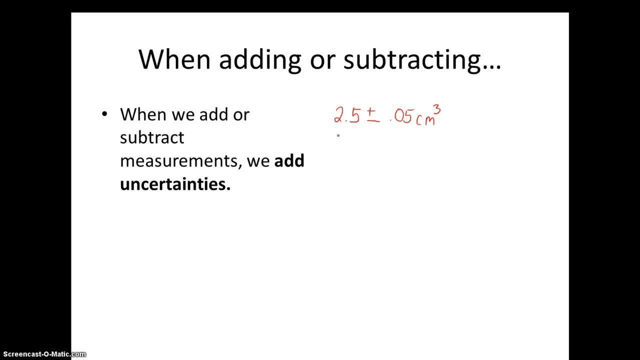 Now I'm going to add that volume of water to another volume of water. This measured value is 5.0 plus or minus .05 cubic centimeters of water, Both of these probably having been measured in a graduated cylinder. I want to add these two values. 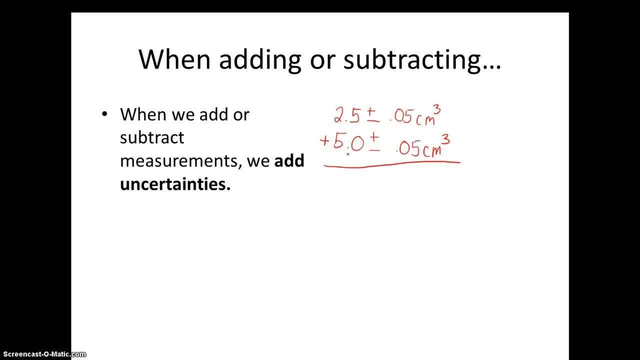 To add them. I'm going to treat first the normal numbers- Normal being just the ones that haven't been messed with in any sort of uncertainty- And I'll add them. normally You get 7.5, and that's beautiful. My significant figures are fine. 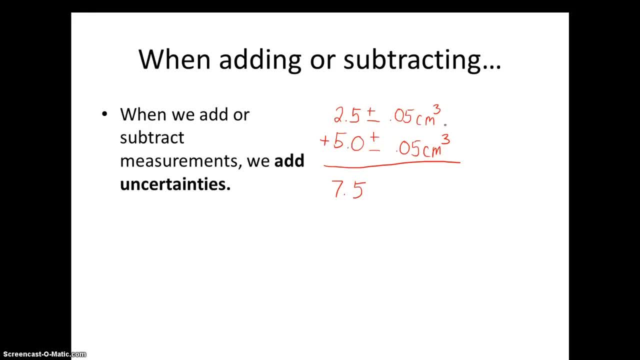 There's nothing to worry about there. And then I will also add my uncertainties. I still keep the plus or minus, But .05 and .05 add up to be .1 centimeter cubed. You'll notice I didn't write .10, because that would be two significant figures. I only want one significant figure, But this is how I'm going to go about adding these values: .05 and .05.. The same thing is true if I subtract measurements. I'm going to treat it the same way. So let's see how that works. 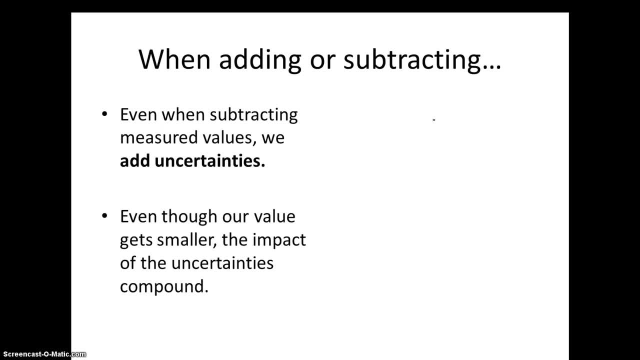 When we're subtracting measurements, we're still going to add our uncertainty, The idea being that, even though our number values may get smaller, the overall amount of uncertainty increases when we put those two numbers together. So we're going to add uncertainties even if we're subtracting other numbers. 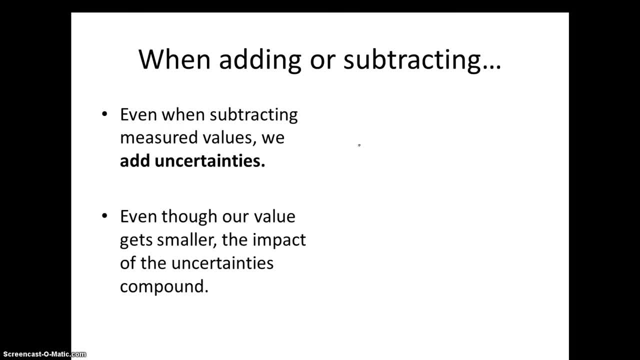 So here's an example. Let's say I've got a mass of filter paper at the end of my lab- 5.23.. I've got a good decimal so that we're all happy with it, And plus or minus .005 grams is the measurement that I managed to get out of our digital balance. 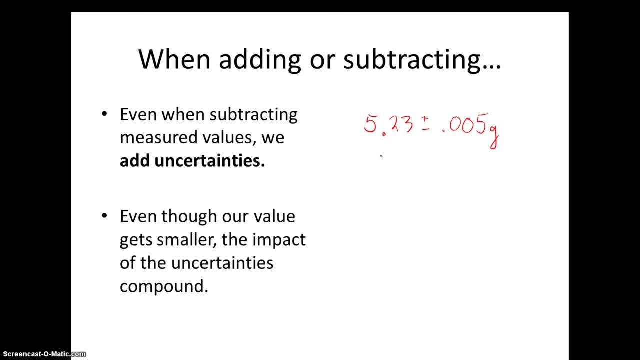 So that's a nice measurement to finish a lab with. It looks all pretty. I measured the initial mass of that piece of filter paper as 4.22 plus or minus .005 grams at the start of my experiment. In other words, my filter paper has gained weight. 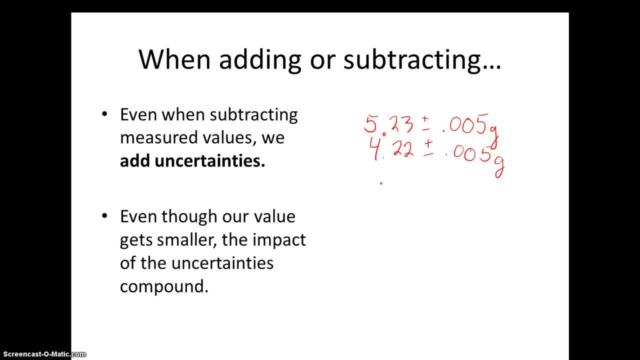 This makes sense because it's filtered some sort of material out, hopefully. That's why we use it Now to figure out how much material is on that filter paper. all I have to do is subtract these values. I have my starting value and my ending value. 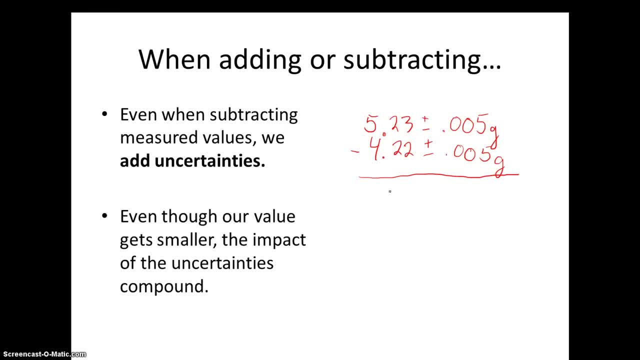 Set up my little math problem. I'll plug it into a calculator. I deal with the normal parts of the number first: 1, 0, 1.. That's beautiful. I just subtract it as normal. However, my uncertainties aren't subtracting from each other. 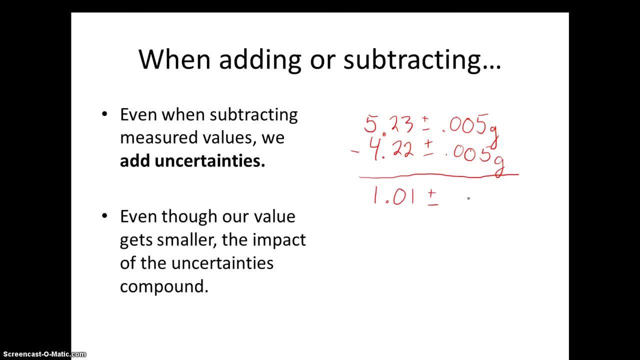 If I did that, I would be saying that I had no uncertainty at all. That's ridiculous. I can't take two measurements that are uncertain, plug them into a calculator and suddenly eliminate the reality from it. What I need to do is make sure that my reality. 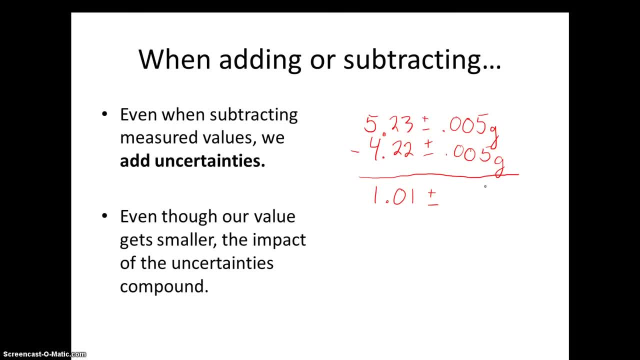 is reflected. I'm taking an uncertainty and I'm applying another uncertainty to it. Those are additive, So my uncertainty in this case becomes 0.01.. And then I'll label my unit 1.01, give or take 0.01 grams. 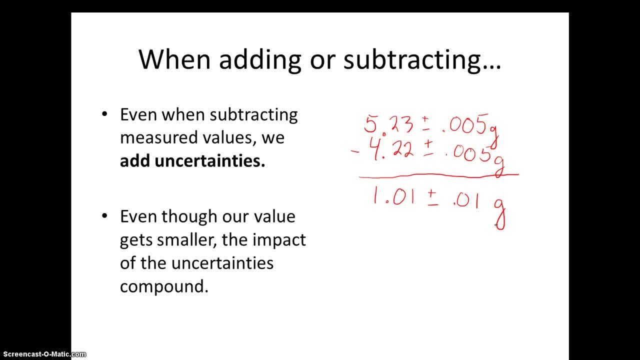 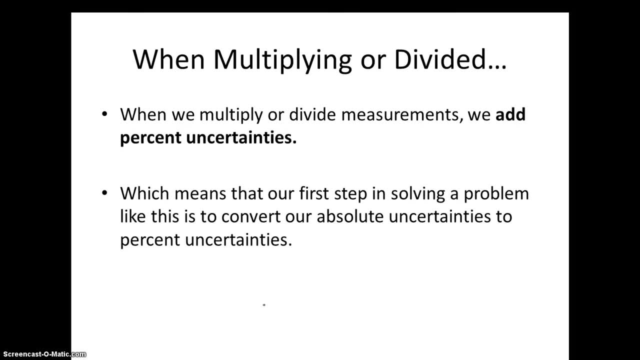 becomes a very reasonable uncertainty to work with here. So that's how we handle adding and subtracting uncertainties. Next we're going to look at multiplying and dividing. When we multiply or divide measurements, we add uncertain. Let's try that again. 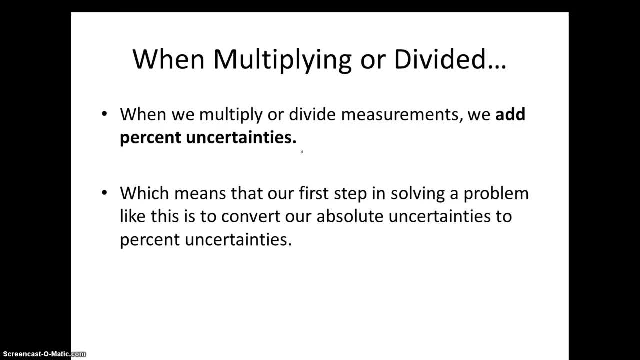 When we multiply or divide measurements, we add percent uncertainties. When we've had our measurements before, we're dealing with absolute uncertainties. We are absolutely 0.1 gram above or below give or take in that range. In order for us to multiply and divide, we need to create percent uncertainties. 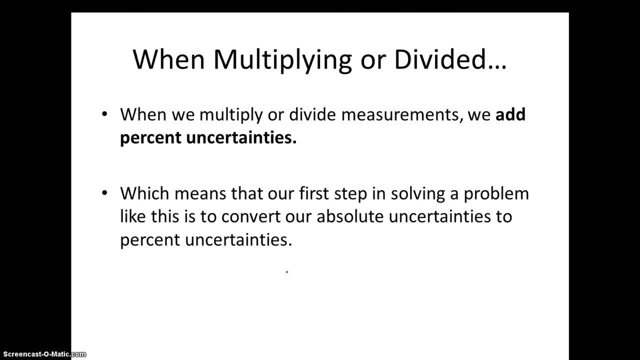 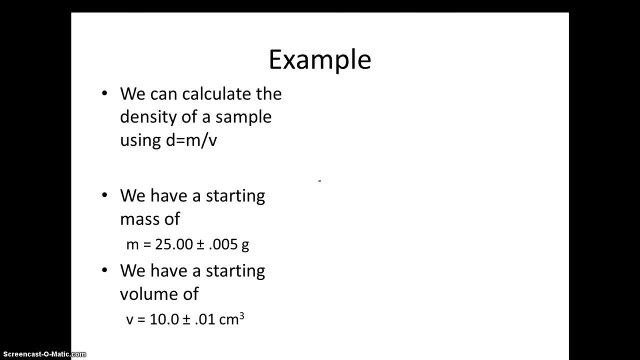 If those don't come from measuring, we have to calculate those percents to work with. So let's give that a try. For this stage, I've picked a density calculation to work with. It's a simple formula that involves division of a mass divided by a volume. 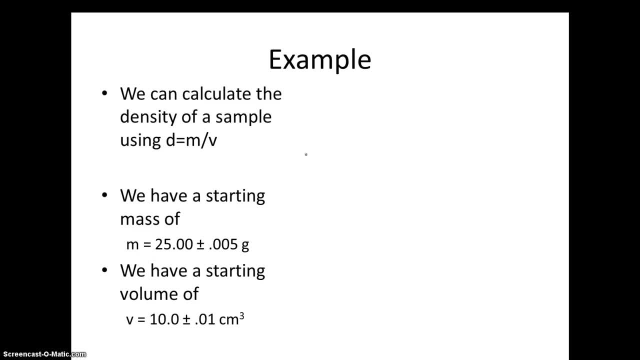 So we can calculate the density of a sample using. density equals mass over volume, And I've picked some starting measurements to work with that are pretty typical of what we might come up with in a lab, except the numbers are really pretty looking. We have a starting mass of 25.00,. 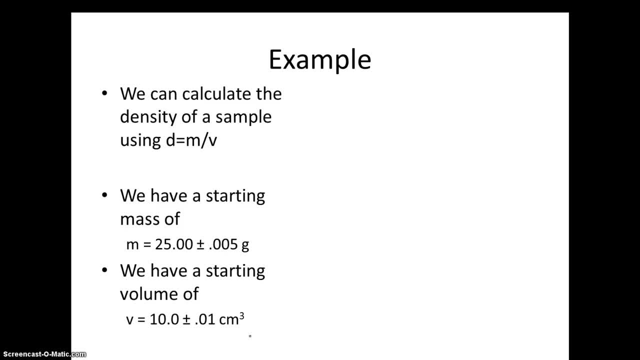 plus or minus 0.005 grams, as we might get off of our digital balance, and a volume measurement of 10.0 plus or minus 0.01 cubic centimeter, as we might get from a graduated cylinder, And I'd like to be able to apply those to our math problem. 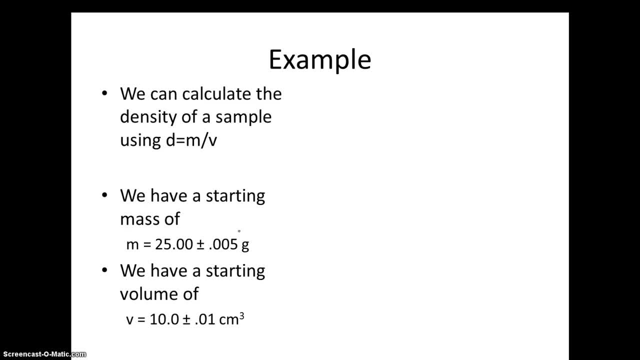 To begin with, I'm going to need to convert my 0.005 gram absolute uncertainty to a percentage. In order to do that, I'll treat it as a percent problem: 0.005 grams divided by 25.00 grams times 100.. 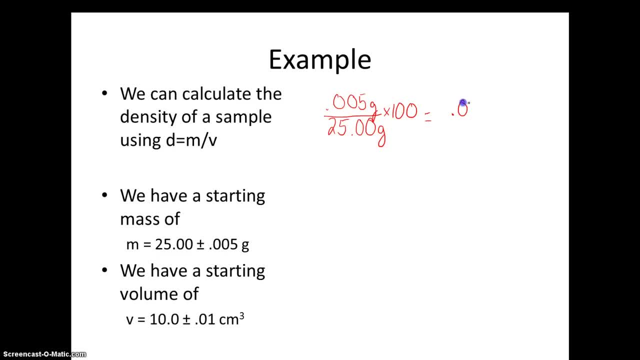 That's a percent problem, And what we get out of that is 0.02 percent uncertainty. Likewise, I'm going to do the same thing for my volume measurement: 0.01 centimeter cubed Divided by my starting amount, my normal value. 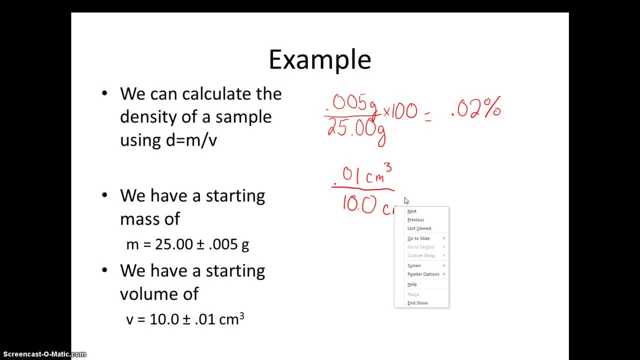 10.0 centimeters cubed. Sorry about that extra button pop up there. Centimeters cubed times 100.. Typical percent problem at this point And that gives me a 0.01 percent uncertainty. So now I can reflect the numbers that I'm working with. 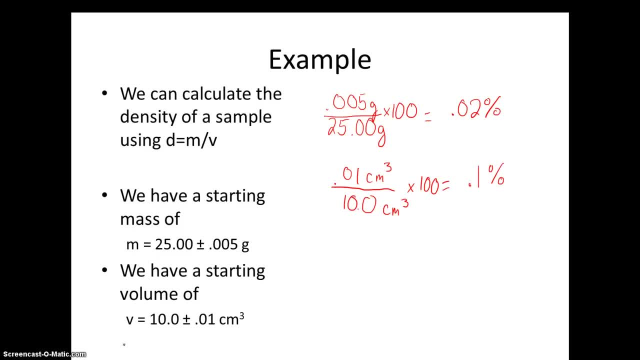 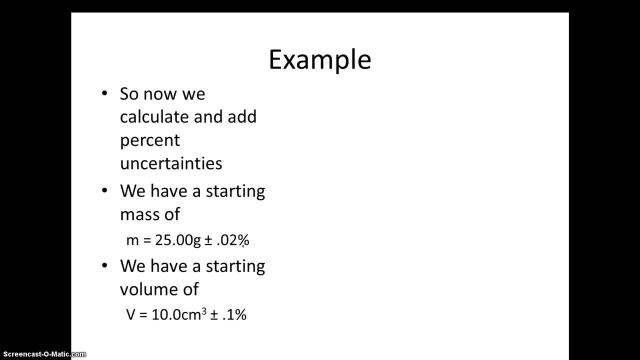 Instead of with absolutes, I can present them with percentages. You'll notice I'm reflecting my measurements here as percentages. Just change that, And now we'll be able to add them when we're doing our math. Let me set this up for you. 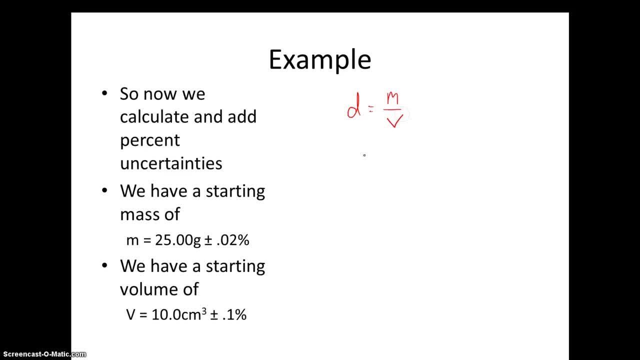 Density is mass divided by volume. My density, then, can be calculated as 25.00 grams divided by 10.0 cubic centimeters, And we handle the normal numbers without their uncertainties, just as we would handle any other little problem in our calculator. 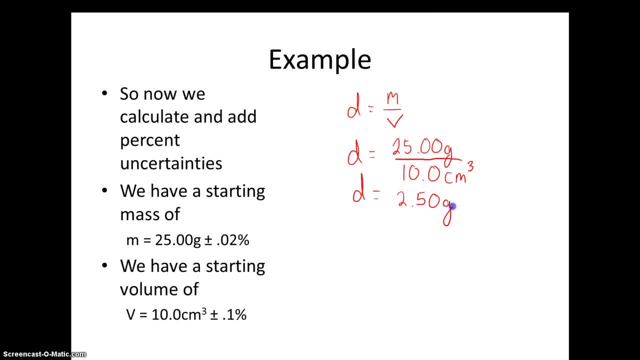 We get 2.50 grams per cubic centimeter And we'll clean that up later because we know IB doesn't like that format. So 2.50 grams per cubic centimeter. For the uncertainties, we add them. I'm going to add 0.02 and 0.1 as percentages. 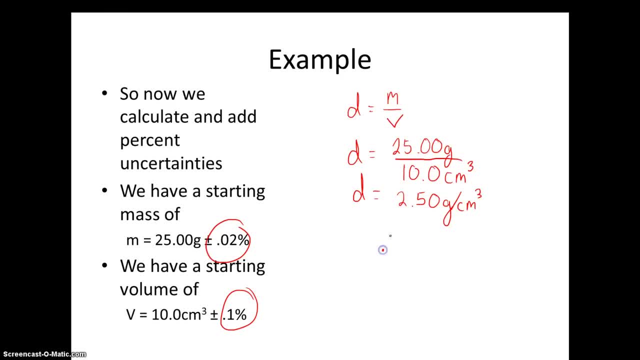 So that my uncertainty percentage here is 0.12 percent- Give or take or plus or minus. So I could report an answer right now of 2.50 grams centimeters to the negative. third: Give or take, plus or minus 0.12 percent. 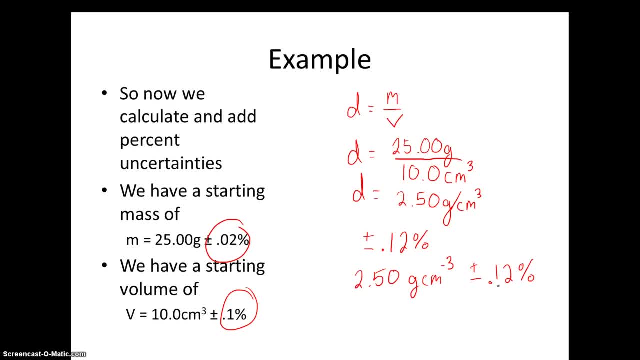 But we typically won't leave it like this. There are two problems. One, I've got too many significant figures here, And two, I've got a percent And that's not really practical for us to use in the lab. So the next step is going to be converting that percent back into an absolute measurement. 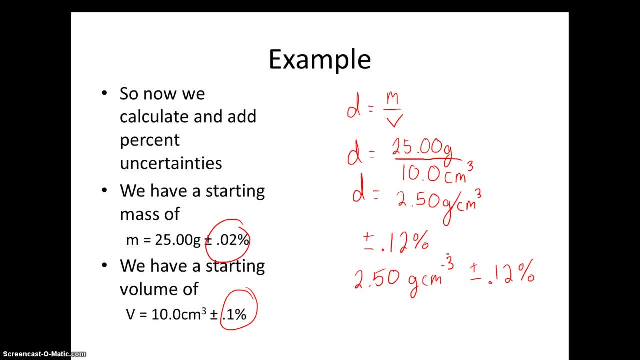 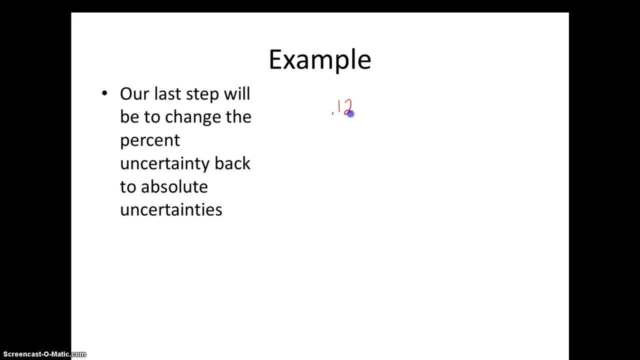 And we'll do that by taking a typical percent problem. Find out what 0.12 percent of 2.50 grams per cubic centimeter happens to be. So let's make that happen. I've got 0.12 percent of my amount, 2.50 grams. 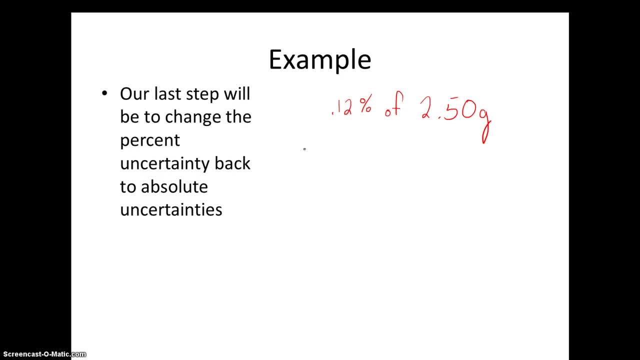 And if I want to take 0.12 percent of this, I'm going to set up a multiplication problem- 0.012 times 2.50 grams- And we'll calculate that amount to get our absolute measurement Thanks to a handy dandy calculator. 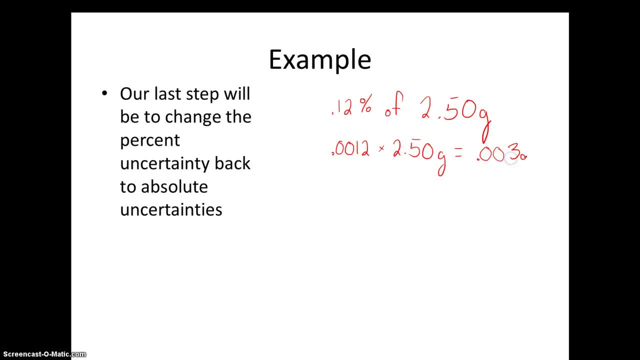 we can figure out that this is 0.003 grams, And now I'll be able to reflect my answer with an absolute measurement of 2.50 grams, plus or minus 0.003 grams. Not too shabby, We're back to an absolute. 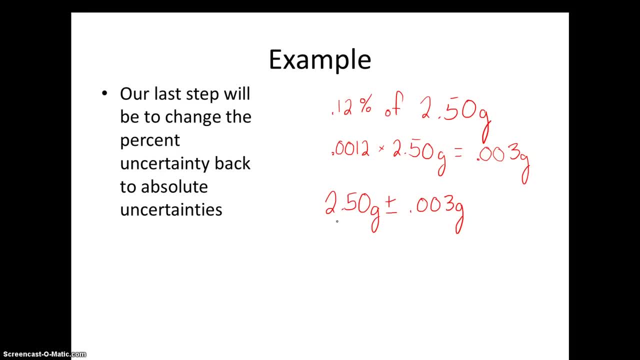 We've only got one sig fig. We've got a mathematically valid answer that reflects the uncertainty. I know it's a lot of work dealing with the percentages in there, But it's worth the effort to be as accurate as humanly possible. 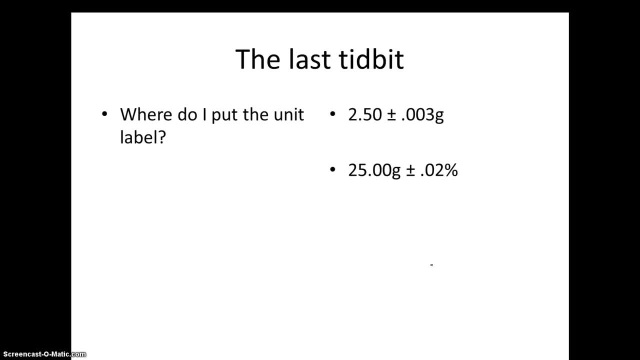 One last little tidbit to talk about: Where do we put the unit label? You've seen me put it in a couple different places. Now, the truth is there's still a little bit of debate about where the right spot should be, Typically what I've run across and what I prefer to do.